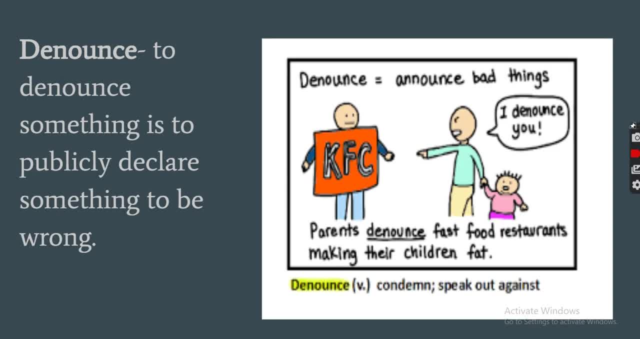 derision kind of mocking attitude. The next one is denounce and denounce. to say something publicly that's negative or declare something's wrong, just like this cartoon here. You know, I denounce you because KFC makes fast food, restaurants make our children fat. 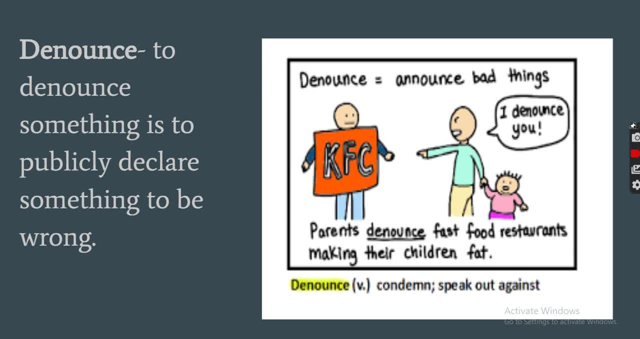 Well, is that true? No, because you took your kids to there. but they're publicly denouncing, you're the problem. And so, in satire, they'll say: oh well, so-and-so is the problem. and they'll publicly say that's a problem, but they're really making fun of them. 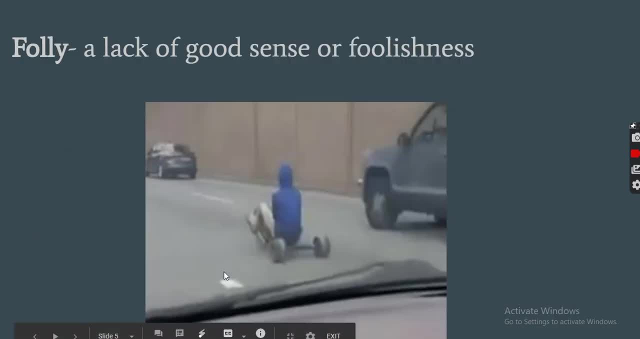 The next one is is folly and that's just a lack of good sense. So here we have, here in this clip, a fool riding- and I can't say it any other way- a fool riding a tricycle down the middle of a. 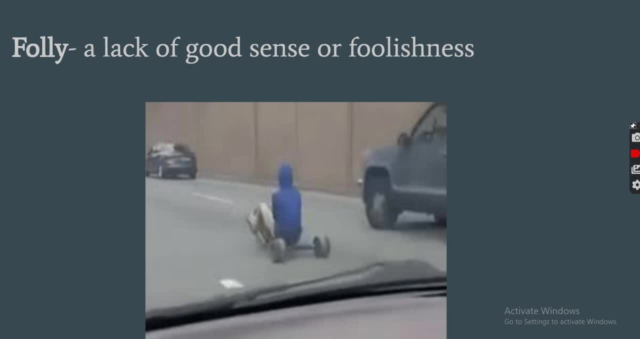 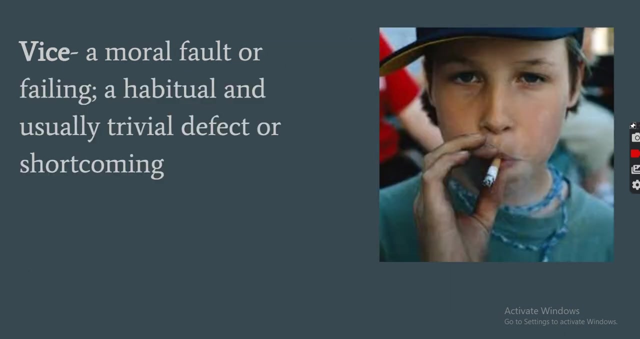 highway. Here he is Now. is it absolutely stupid? Yes, Is it foolish? So that is a folly. So if something is just lacks good sense or is absolutely stupid, then it's a folly. So if it's absolutely foolishness, that's called a folly right. The next is a vice and that's a moral. 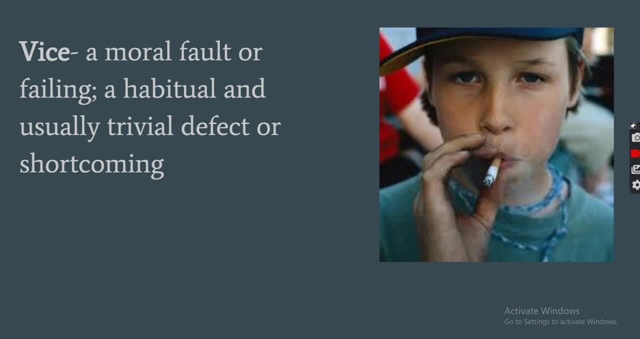 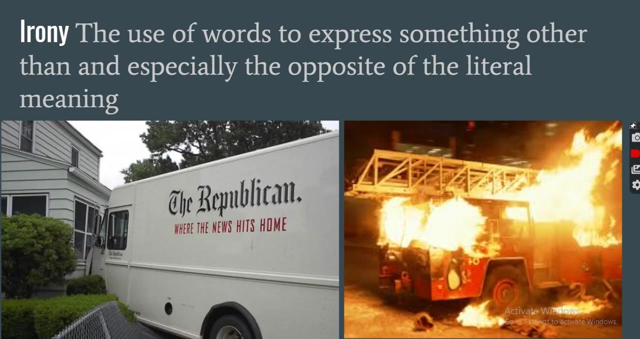 fault or fail or failing like a habit. So here's a vice: a child smoking a cigarette, That's a vice. We know that shouldn't happen, So that's called a vice, right? The next one is irony and I love. 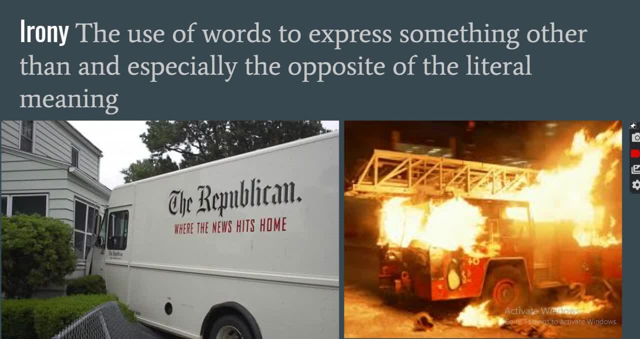 irony, Irony. Irony is the use of words to express something other than, and especially the opposite of, literal meaning. Here we have this delivery truck, the Republic, which is a newsstand where the news hits home. It literally hit home. Or we have a fire truck on fire. The irony is: 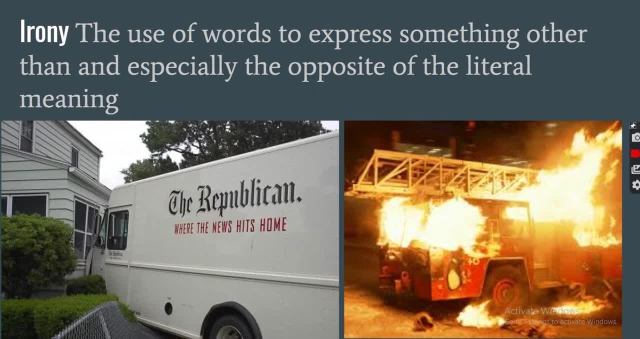 the truck shouldn't be hitting the home and a fire truck shouldn't be on fire. but you see it, You see it's called irony because it shouldn't be, but it is kind of happening. We see irony a lot, So you could say one thing, but it really means something else, almost just the opposite of it. 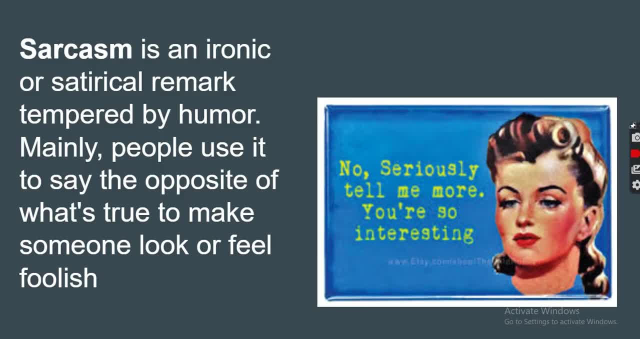 right, And then we've got sarcasm. Now, this is a language you guys know already, but I put it in anyway. It's using that remark or humor that you're trying to make fun of someone, And so I pull this one up, because this one sounds more like y'all. No, seriously, tell me more You're. 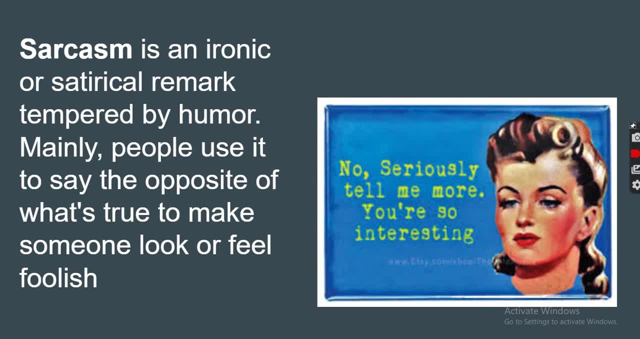 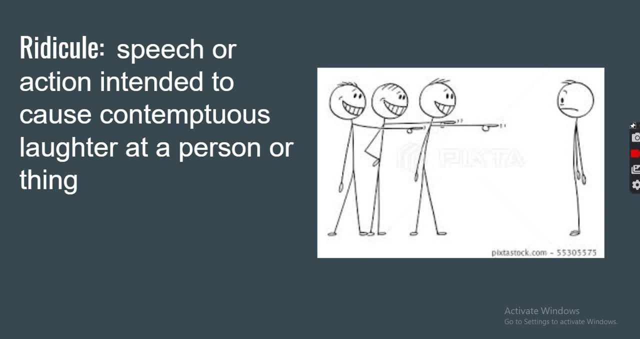 so interesting And so sarcasm you guys will not have a problem finding. The next is ridicule, and that's another one You shouldn't have any problem finding, and that is speech or action or anything that is pointing laughter at one particular person or a thing. 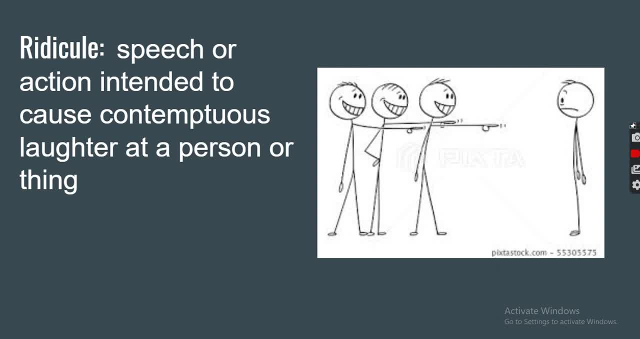 And so here are these. you know, these people are pointing and laughing at this one person, and that's called ridiculing them. Now, here's what I want you to do. We have. we have all of these things that you ought to have. 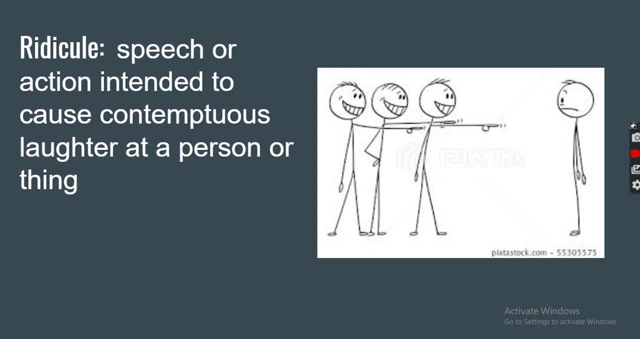 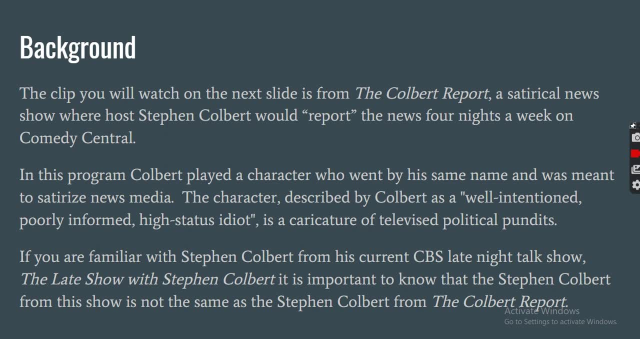 in your notes and you can play it back at them, to your notes. Then what I'm going to want you to do is I'm going to want you to watch a video. Now, let me give you some background on this video. This is the Colbert Report. Now, so you understand who Stephen Colbert? 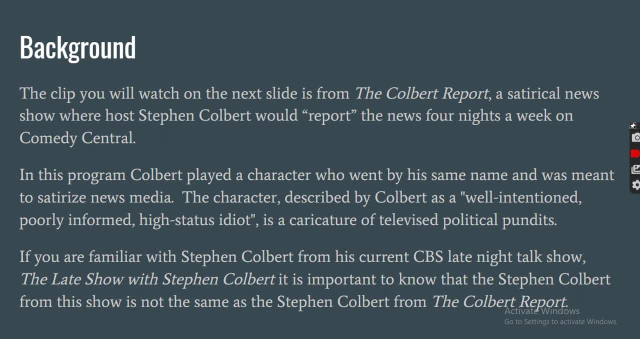 where he is. Stephen Colbert started doing this program inside of a program and he did this program. He was a character in the program and it says here in the middle paragraph: he was well intentioned, poorly informed, a high status idiot. And so he plays this almost a bumbling kind of guy. 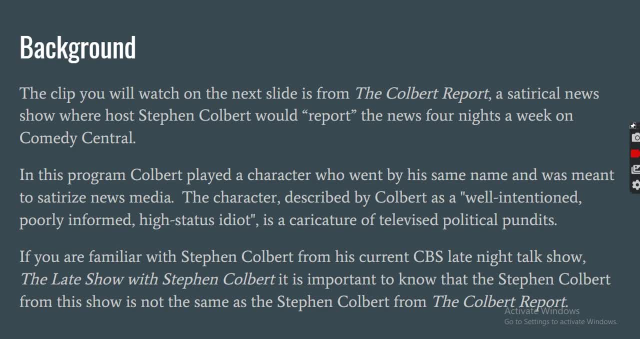 in it. Now you're going to watch a clip from that Now. Stephen Colbert also has a show in CBS. It's called The Late Show with Stephen Colbert. In that he's not playing the idiot, He is just being a talk show host. But in this was one of his first things. He did this, Stephen.